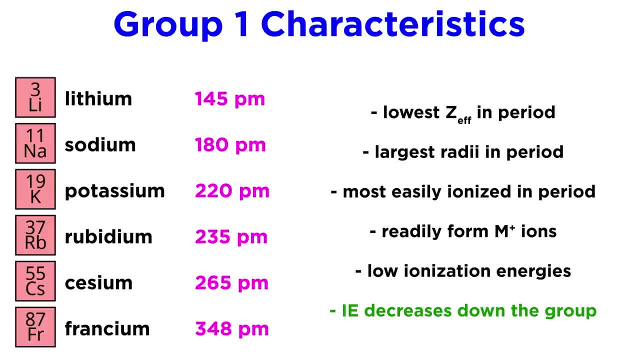 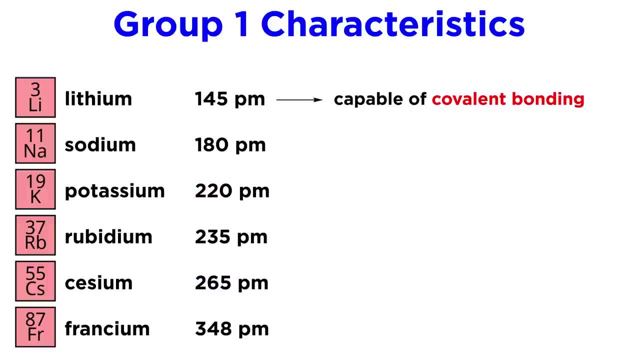 additional shells and the valence electron gets farther and farther from the nucleus. Lithium is the only element in this group that is capable of sometimes forming covalent bonds, and this is due to its small size, which results in a strong hold of its electrons. 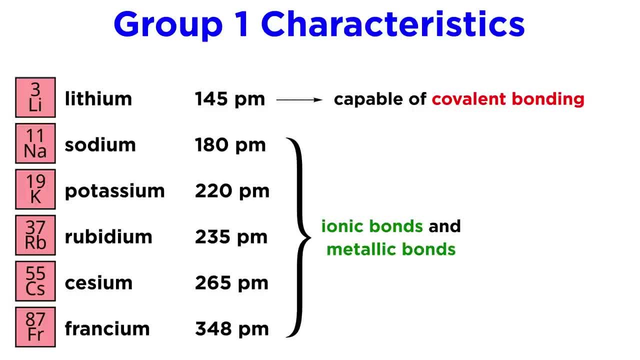 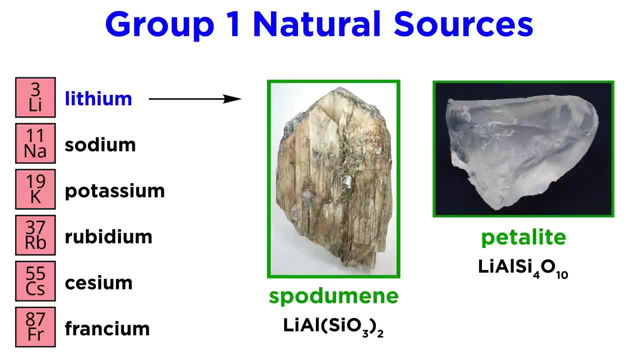 The rest tend to only make ionic bonds and metallic bonds. So where can we find these elements? what are their natural sources? Lithium is derived from ores like spodumene and petalite, Which have the formulas given. Commercial deposits are rare and found mainly in Bolivia. 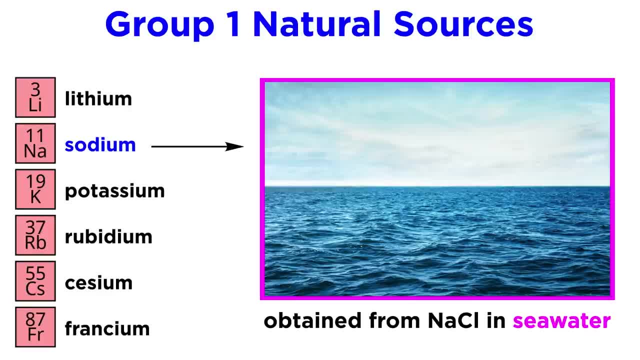 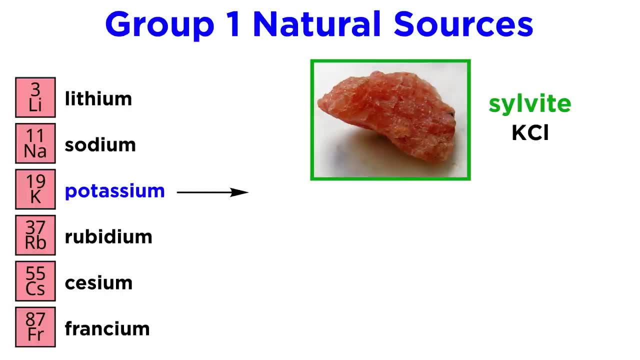 Sodium is obtained from sodium chloride in seawater. The seawater evaporates and produces halite deposits. Potassium is obtained in a similar manner from minerals in seawater that has evaporated. These minerals include sylvite, which is potassium chloride. 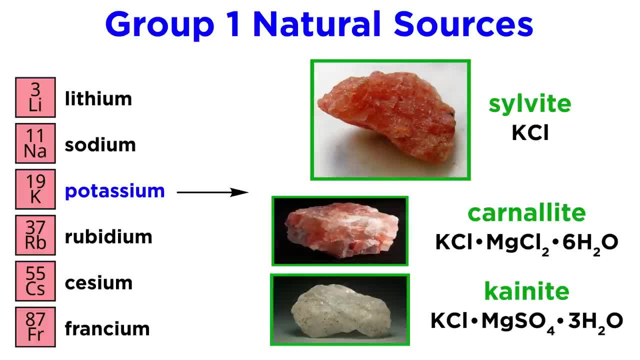 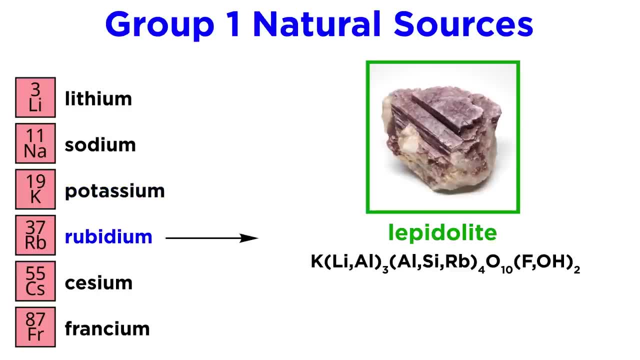 as well as carnalite and cainite, which are hydrates with these structures. Rubidium is found in the ore lepidolite, with this complicated structure where a small amount of potassium is replaced by rubidium. This is found primarily in Brazil. 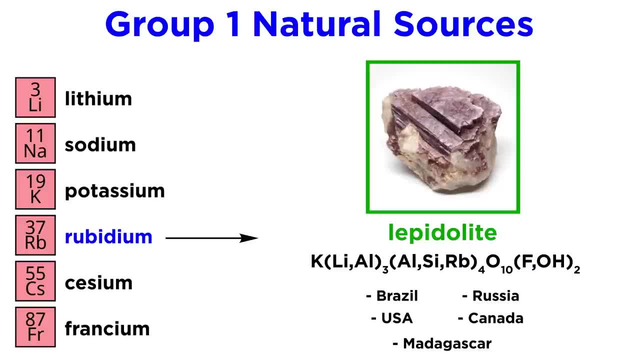 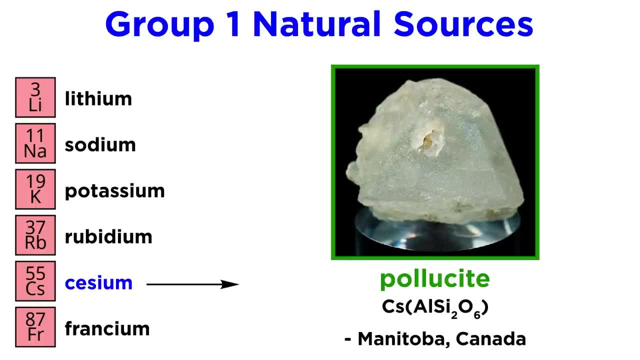 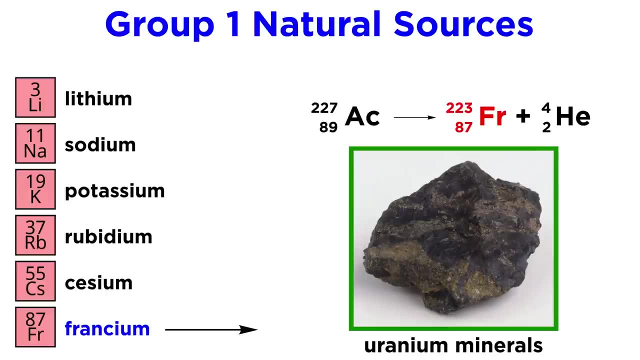 Russia, the United States, Canada and Madagascar. Cesium is found in the ore palusite, which is found primarily in the Manitoba province of Canada. Francium is exceptionally rare, formed as the result of radiation and is a radioactive decay of actinium which occurs in uranium minerals. All of Earth's crust. 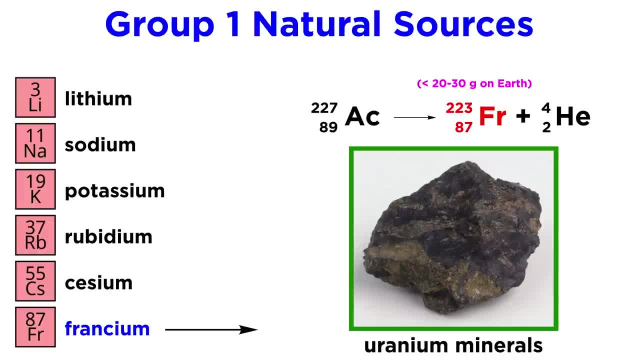 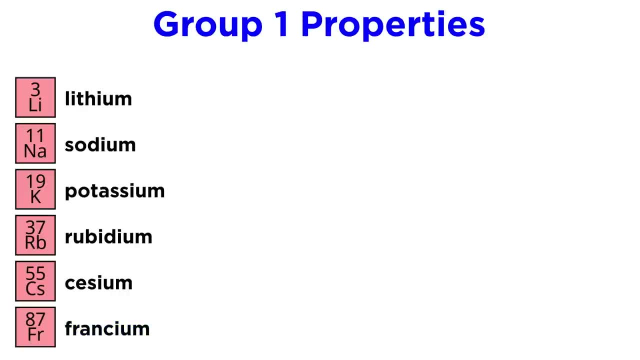 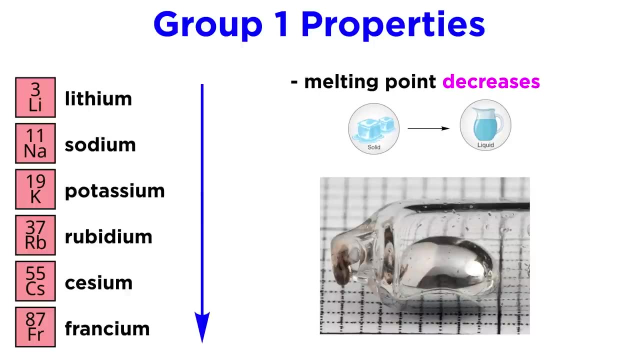 probably contains less than 20-30 grams of francium at any given time. Francium can also be made artificially in particle accelerators. Now a bit on the properties of these elements. Their melting points decrease going down the group, though they are quite low in general. 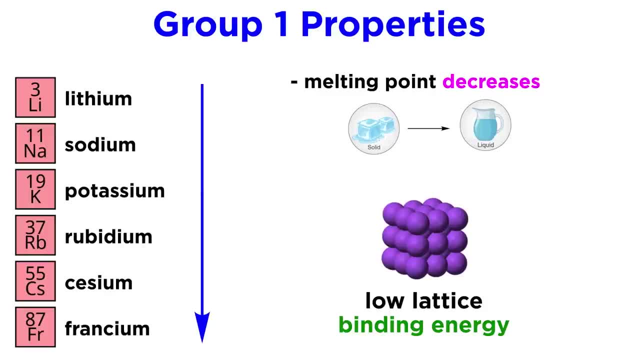 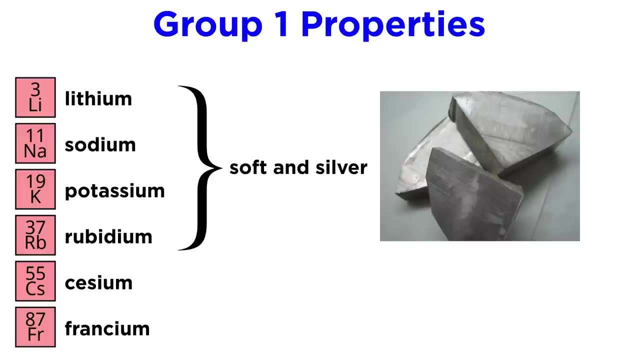 as far as metals are concerned, given the low lattice binding energies that result from having only one valence, electron. The same trend can be applied to their heats of sublimation and hydration energies. Lithium, sodium, potassium and rubidium are all soft and silver, while cesium 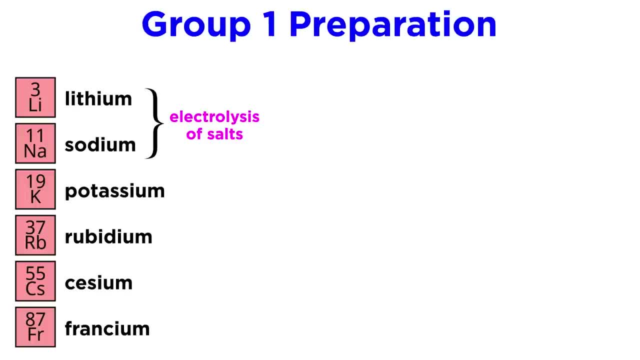 has a gold sheen. In terms of preparation, lithium and sodium can be prepared via electrolysis of salts. Molten sodium chloride will undergo reduction to form liquid sodium and chloride ions. Potassium, rubidium and cesium can be prepared by treating their respective. 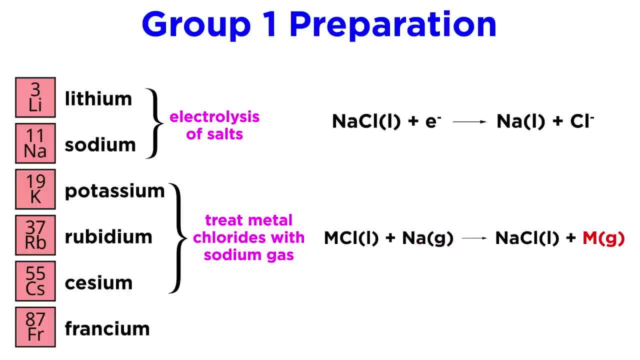 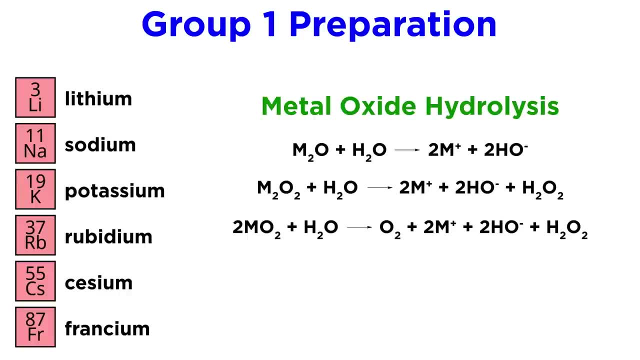 metal chlorides with sodium gas. These are then purified by distillation. Additionally, these metal oxides can undergo hydrolysis to yield metal cations, hydroxide ions and, in some cases, hydrogen peroxide and oxygen gas. Due to their high reactivities, these metals 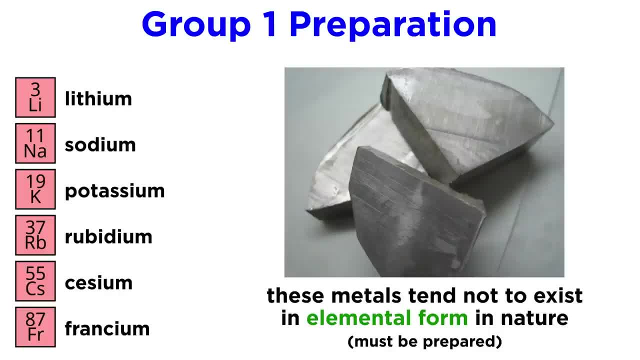 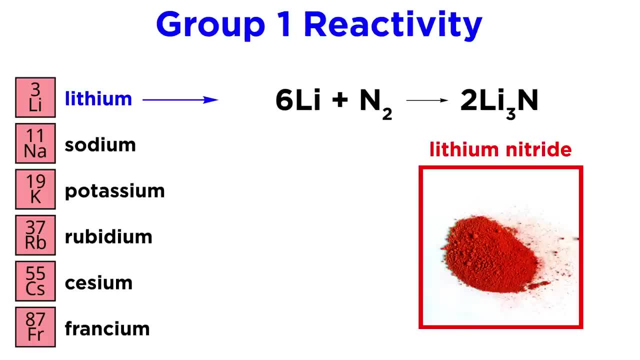 tend not to exist in pure elemental form in nature, which is what makes their preparation necessary. Now, moving on to reactivity. At modest temperatures, lithium reacts uniquely with nitrogen gas to form lithium nitride, a ruby red solid. All the metals react with water to form. 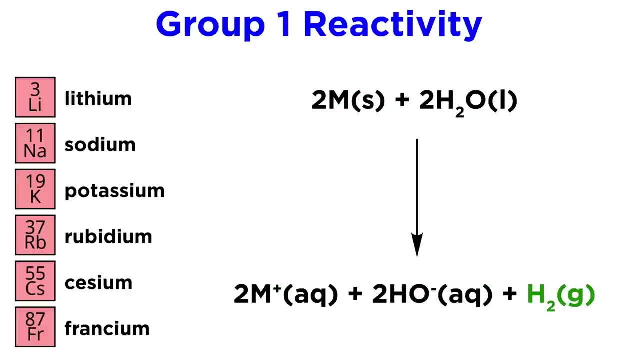 metal cations, hydroxide ions and hydrogen gas. Lithium does so slowly at room temperature, Sodium reacts vigorously, Potassium even more vigorously, while rubidium and cesium react explosively. Again. this is due to the decreasing ionization energy moving down the group. 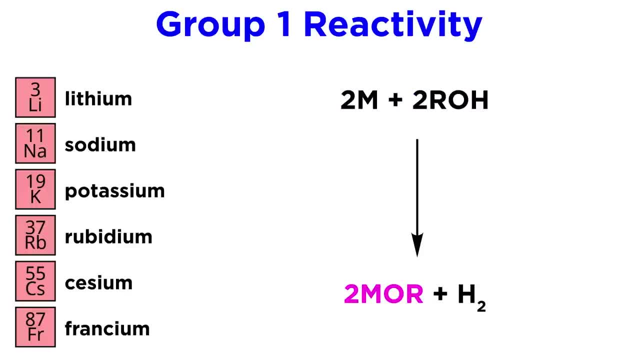 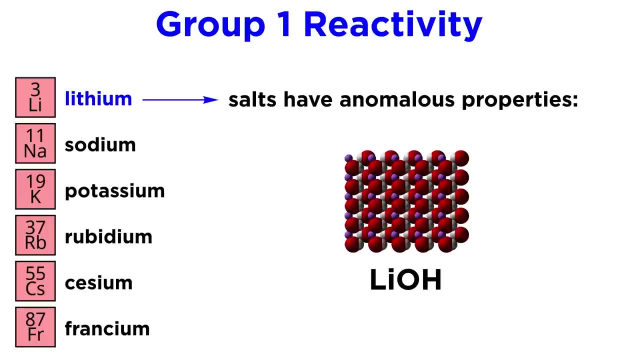 These metals also react with alcohols to produce metal alkoxides. A variety of other salts are also possible. Lithium salts have anomalous properties due to the very small size of the lithium cation. Lithium hydroxide decomposes to lithium nitride. 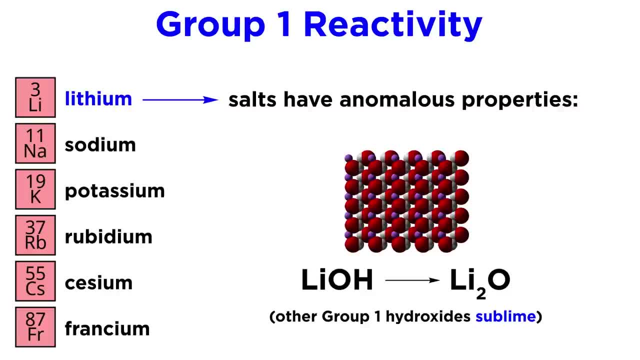 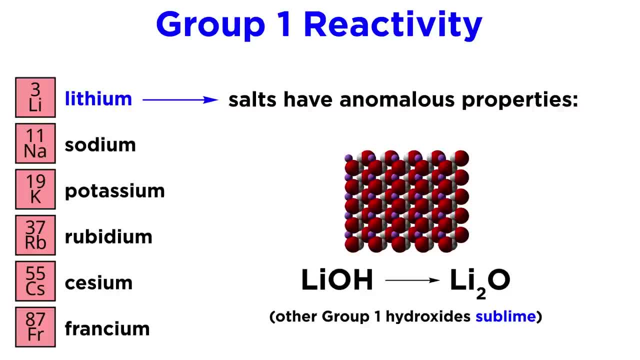 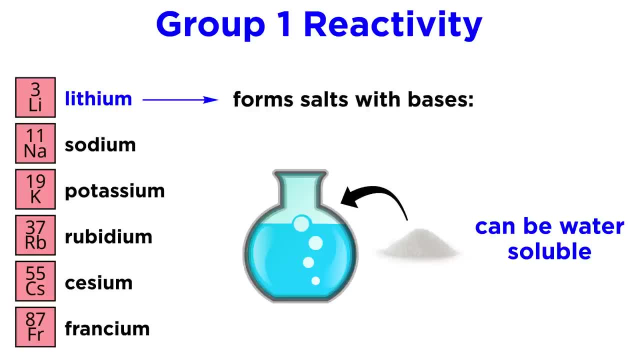 while other alkali metal hydroxides, sublime Lithium forms salts with halides that are soluble in organic solvents. It can form salts with the conjugate basis of Bronsted-Lowry acids that are water-soluble to varying degrees. If derived from a strong acid, the salt is very. 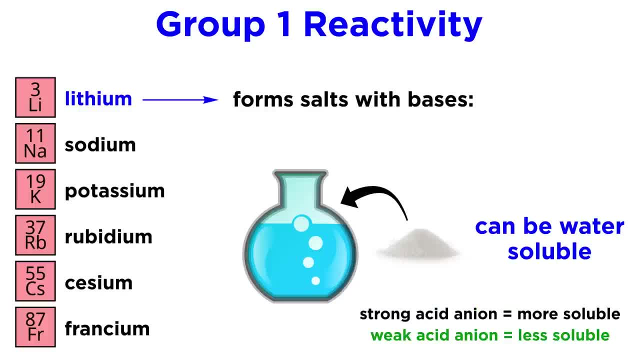 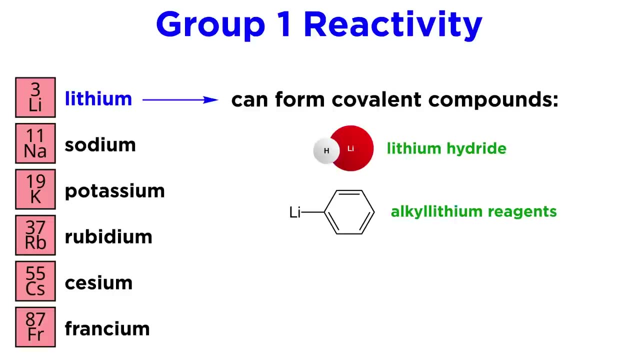 soluble due to the mismatch of ion size. If derived from a weak acid, the salt is less soluble because of the strong bonding in the crystal lattice, which outweighs the energy released in solvation. Lithium hydride is covalent, as are alkyl-lithium reagents, which we learned about in. 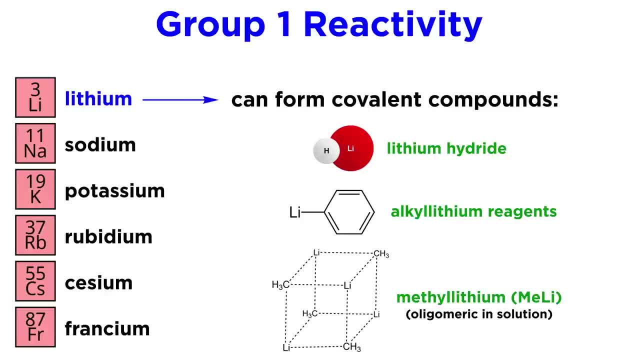 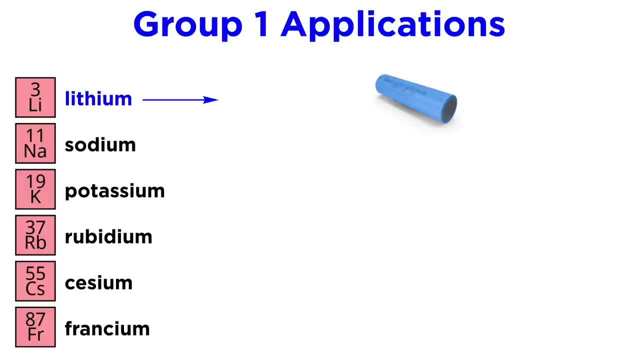 organic chemistry. Methyl lithium is actually a discrete tetramer when in the solid form. Let's now examine some applications. Lithium has tremendous utility in batteries. It is very light and, in fact, at 0.5 grams per cubic centimeter. Lithium has tremendous utility in batteries. It is. 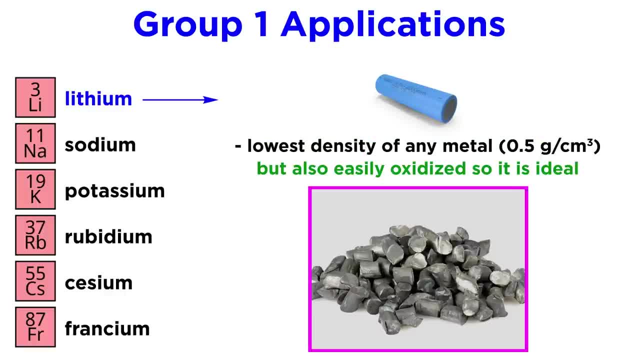 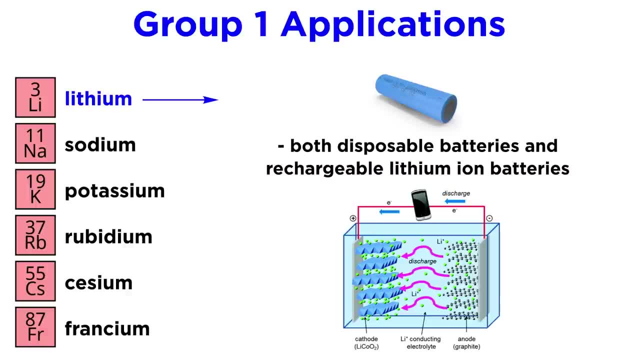 very light and in fact, at 0.5 grams per cubic centimeter, It has the lowest density of any metal, but it is also easily oxidized, so it is an ideal substance. Lithium is present in certain disposable batteries, as well as rechargeable lithium ion batteries, some of which utilize 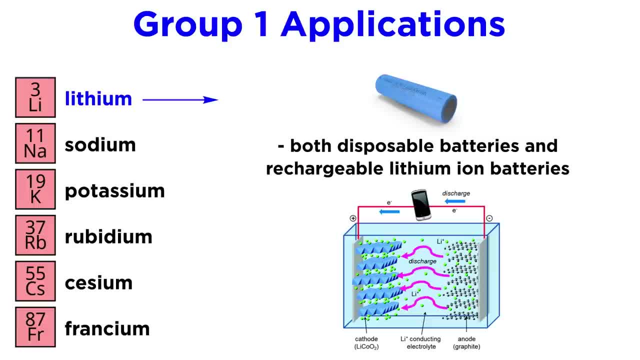 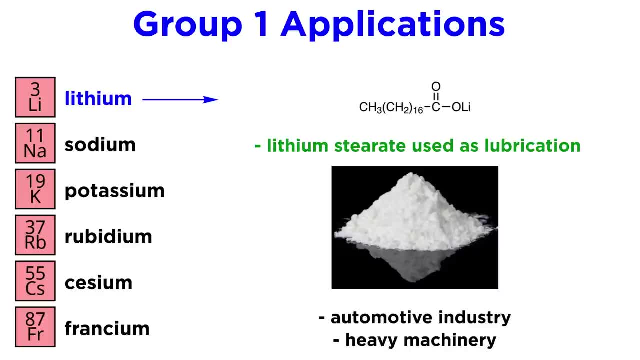 lithium ions that intercalate or penetrate a lattice of cobalt oxide and graphite. Lithium stearate is used in lithium grease for lubrication in the automotive industry and heavy machinery. Lithium stearate is used in lithium grease for lubrication in the automotive industry and heavy machinery. 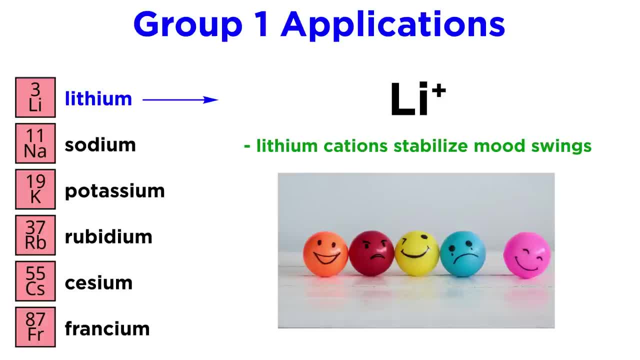 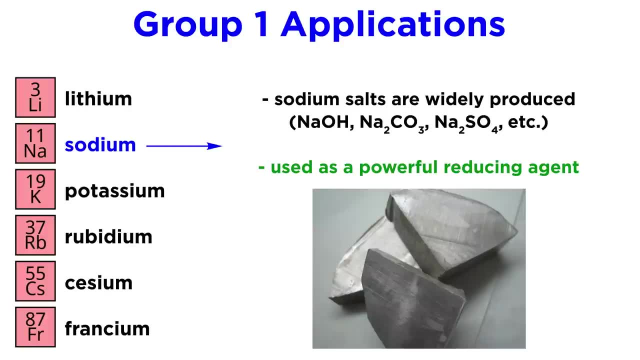 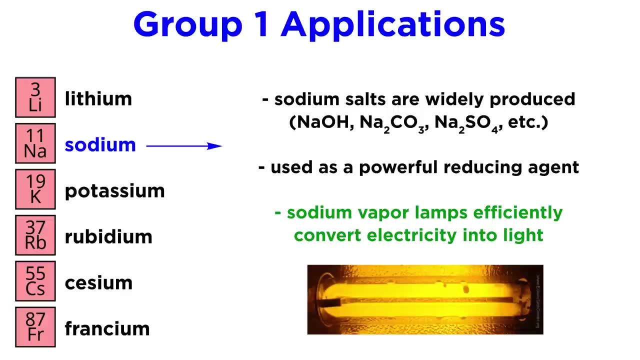 And lithium cations stabilize mood swings in humans. Moving on to sodium, many sodium salts are widely produced. Elemental sodium is a powerful reducing agent. Sodium vapor lamps are efficient at converting electricity to light. Sodium hydroxide is utilized in drain cleaners. 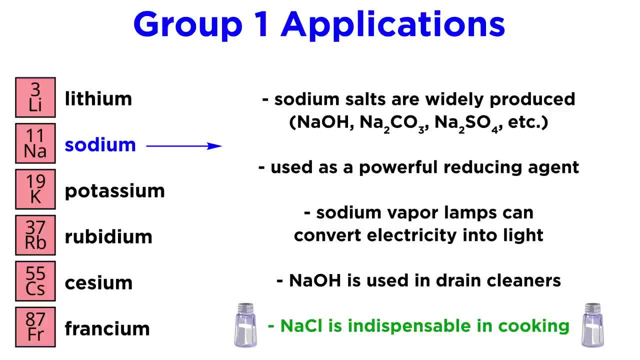 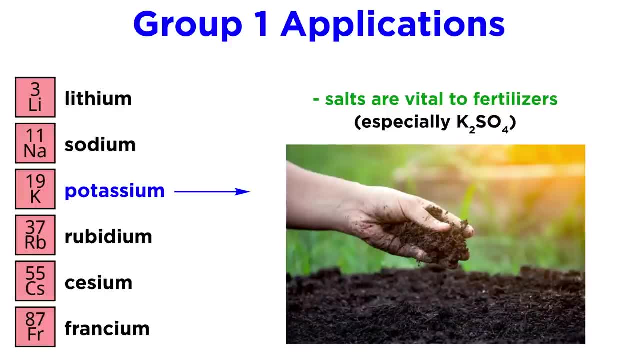 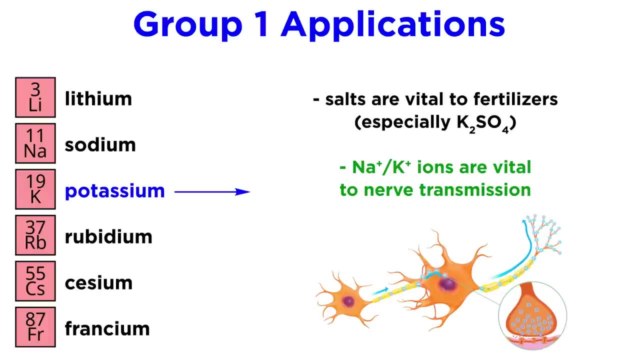 And of course, sodium chloride or table salt is indispensable in virtually every cuisine. Potassium salts are vital to fertilizers. Both sodium and potassium ions are vital to nerve transmission, as we learned about in the biopsychology series. so potassium deficiency. 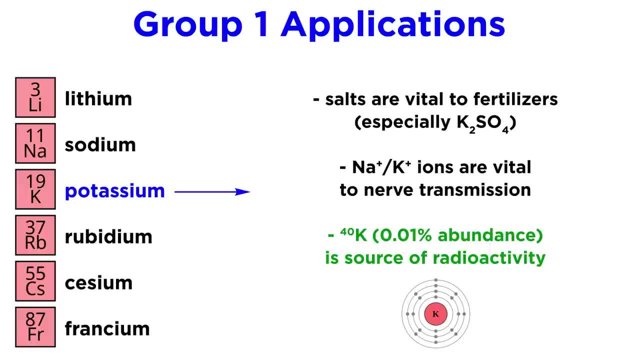 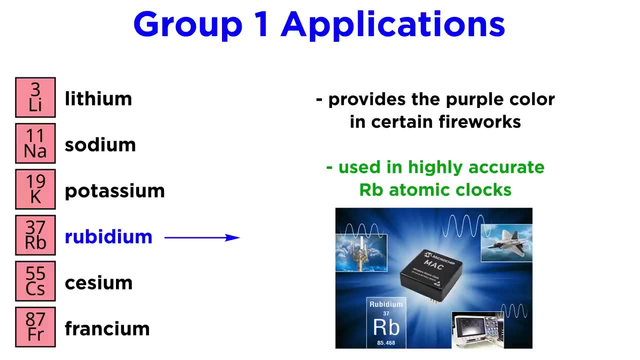 results in progressive paralysis. Also, potassium is a source of radioactivity, as 0.01% of potassium is in the form of the radioactive 40K nuclide. Rubidium provides the purple color in some fireworks. Rubidium atomic clocks utilize a hyperfine transition in its ground state when interacting. 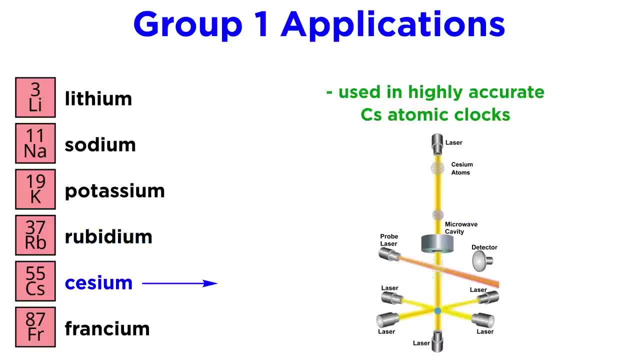 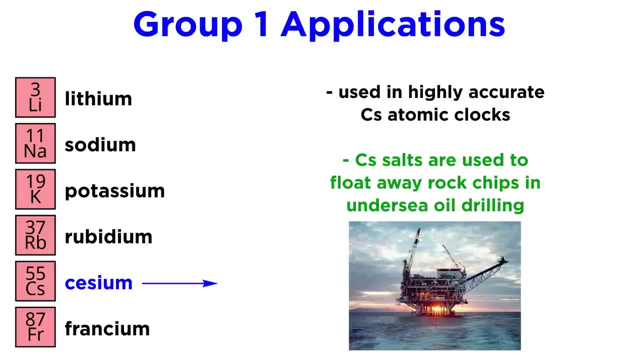 with microwaves, and these are highly accurate. Cesium is also known for atomic clocks. These utilize the same principle as the rubidium variety, but are even more precise, though they are more expensive. Additionally, cesium salts are dense enough to be used to float away.